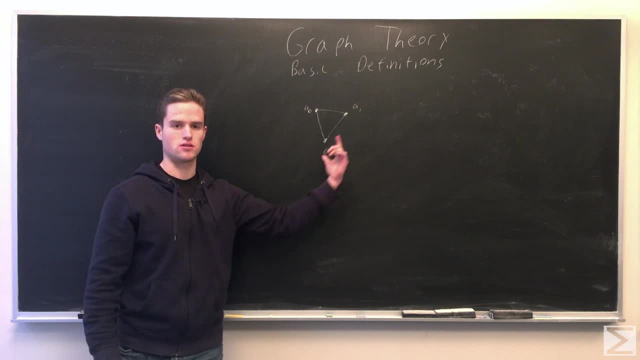 This relation. I call it an edge. There's an edge between these two vertices. So the number of vertices in a graph is the order of the graph. so this has order 3.. The number of edges in a graph is the size of the graph. This has size 3.. 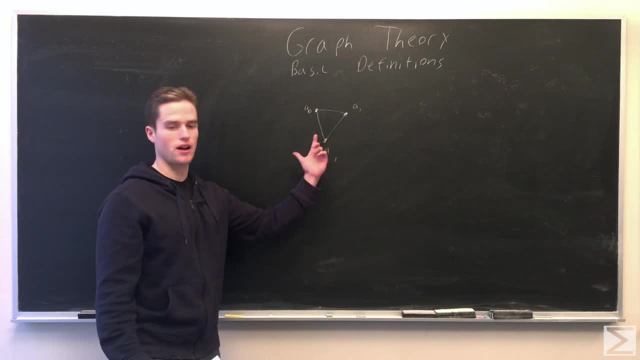 A subgraph of a graph is a graph whose vertices are a subset of some bigger graph and whose edges are a subset of the edge relations of the bigger graph, so say a0 or a2 with the edge between them. this thing would be a subgraph of our triangle here. 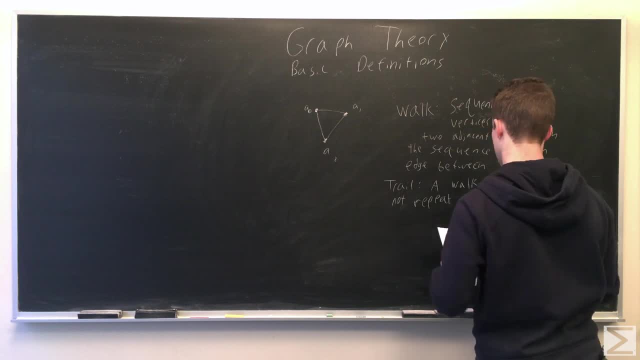 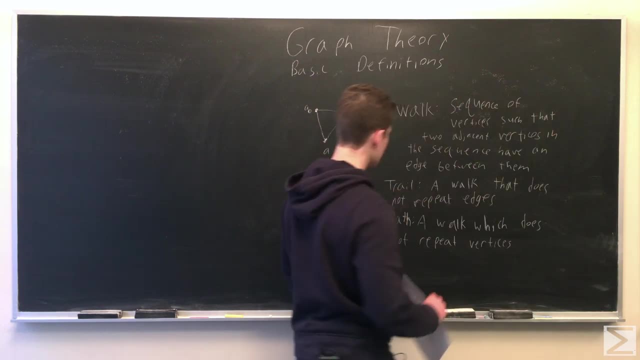 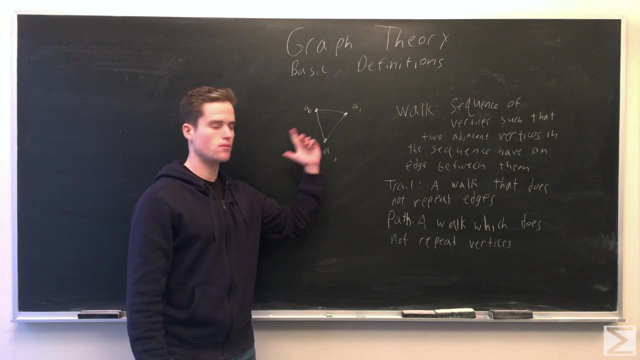 So we have a couple of different. if we have a sequence of vertices, depending on the property of these sequences we can define them differently. So a walk will be a sequence of vertices such that any two adjacent vertices in the sequence have an edge between them. 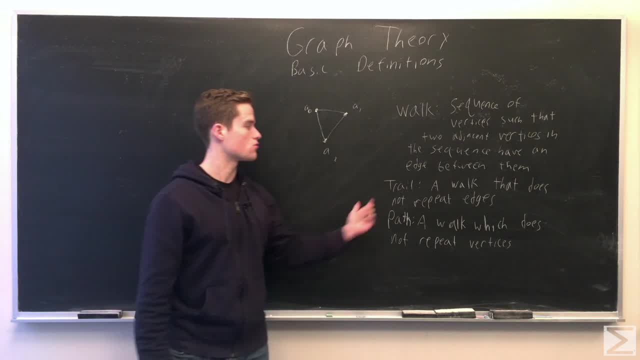 So we're just moving between. We're just moving between vertices in any order we want. A trail has extra restriction. It's a walk that does not repeat any edges, so we go a2, a1.. We're not going back from a1 to a2.. We do not go over the same edge twice. 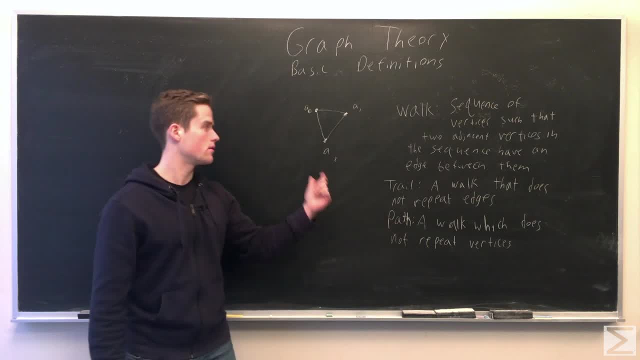 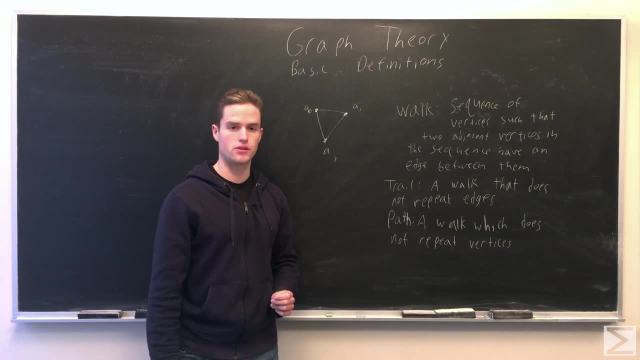 And a path has extra restriction. It's a walk where we do not repeat any vertices. If in the sequence, if we have a trail in which the beginning and end vertices are the same, it's called a circuit. If in the circuit no vertex is repeated, then it's called a cycle. 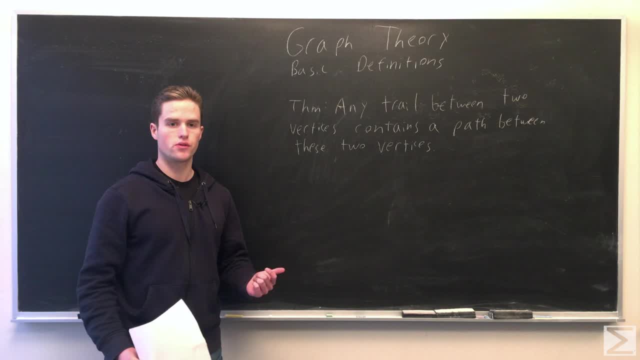 So one thing we can prove is, if we have a trail between two vertices, we can find a sub-sequence from that sequence, such that we then have a path between these vertices. We can find a sub-sequence from that sequence, such that we then have a path between these vertices. 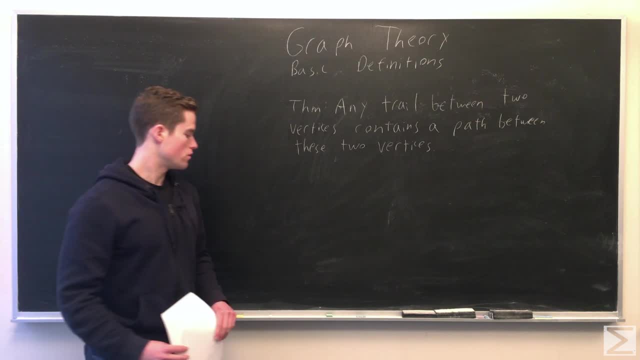 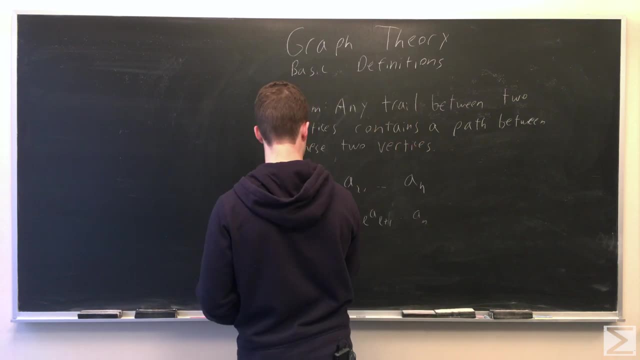 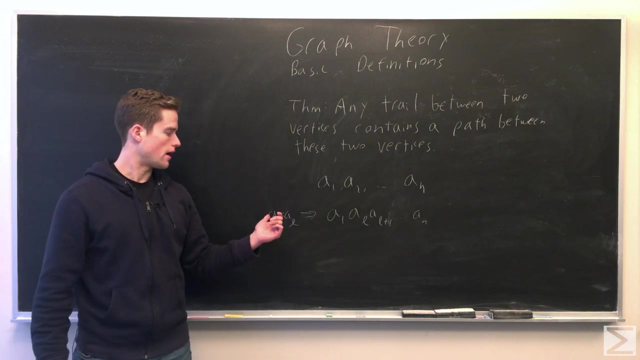 We can find a sub-sequence from that sequence, such that we then have a path between these vertices To do this. So say, we have some trail a1, a2, da-da-da-da a? n If a1, if there's some a l here, that is the last time a1 shows up. 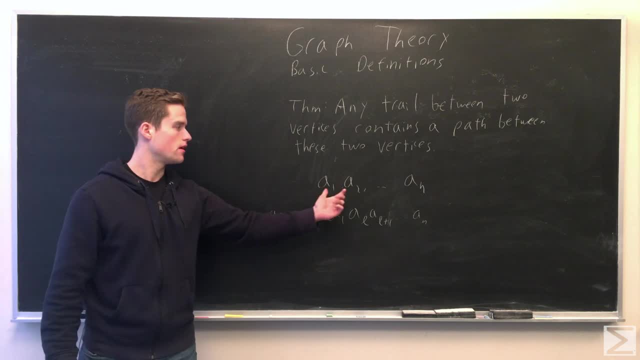 then yeah, so a l is equal to a1.. Then Then remove all the vertices between a1 up to a l. Then remove all the vertices between a1 up to a l. Then remove all the vertices between a1 up to a l. 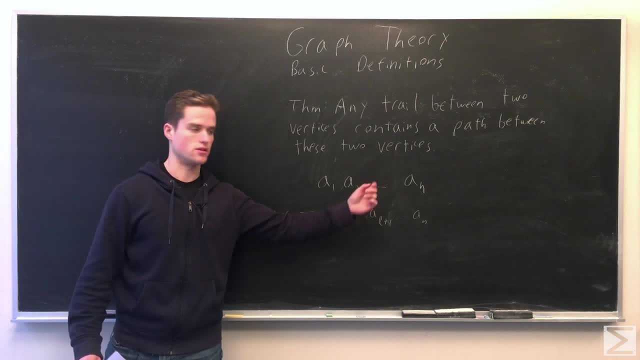 So a2 to a l, remove all these vertices. So a2 to a l, remove all these vertices. And take as a sub-sequence a1, and then the next vertex is a l plus 1, da-da-da. And take as a sub-sequence a1, and then the next vertex is a l plus 1, da-da-da. 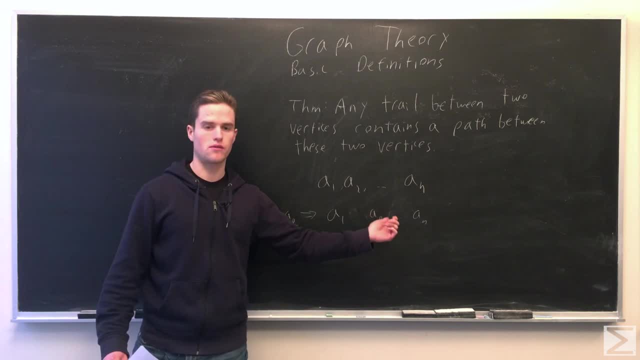 And take as a sub-sequence a1, and then the next vertex is a l plus 1, da-da-da, And then a l plus 1,. do the same thing. find the last time it shows up. remove all those vertices. take the next one. 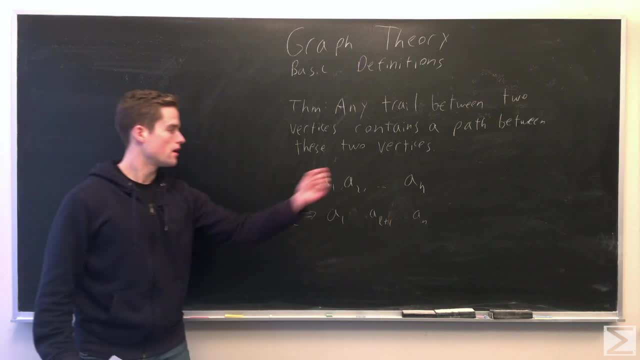 And then a l plus 1, do the same thing. find the last time it shows up, remove all those vertices, take the next one And effectively what we're doing here is, And effectively what we're doing here is. 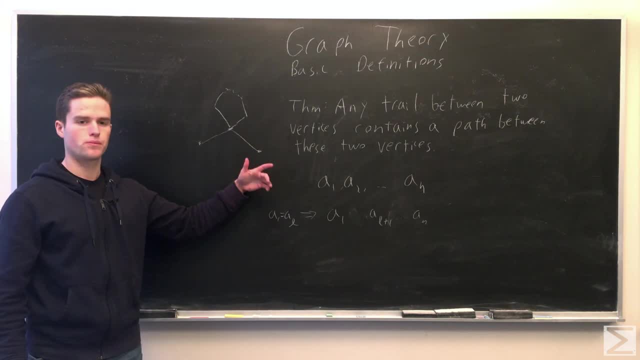 So in our trail, say we start here and at some point we come to another vertex, which something happens, and then we come back to this vertex, which something happens, and then we come back to this vertex. We can remove all these different bits where something is happening. 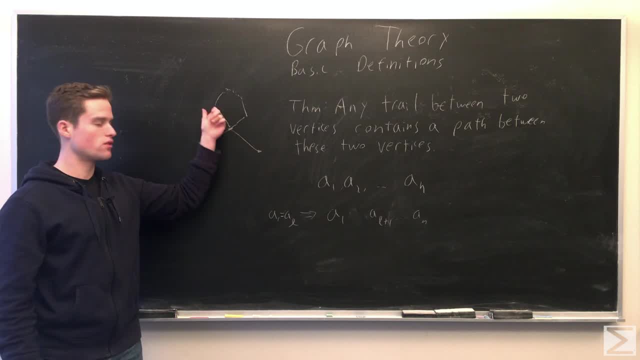 We can remove all these different bits where something is happening, We're not concerned about this. We can just remove this and take as our subset this, this, then the next one, And if we keep doing this, eventually we'll get that each vertex only appears once. 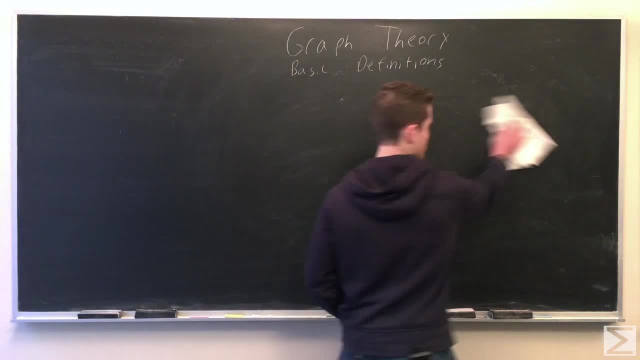 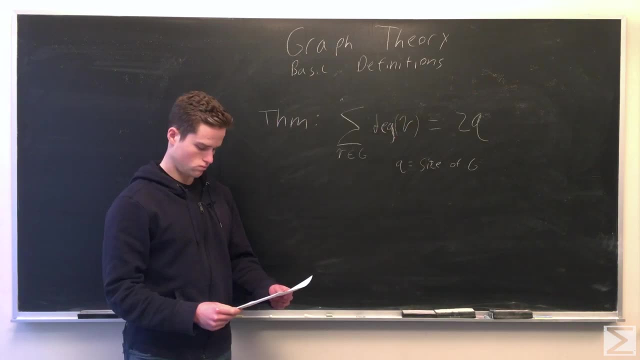 and thus this is a path. So say, we have some arbitrary graph G, we can show N and we're gonna find degree of V. that's for any vertex V. the degree is the number of edges around it, so the number of other vertices. 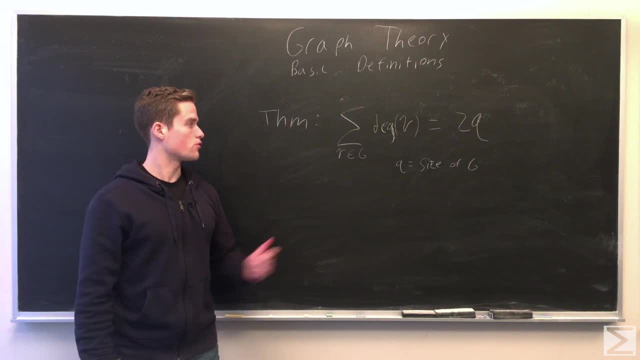 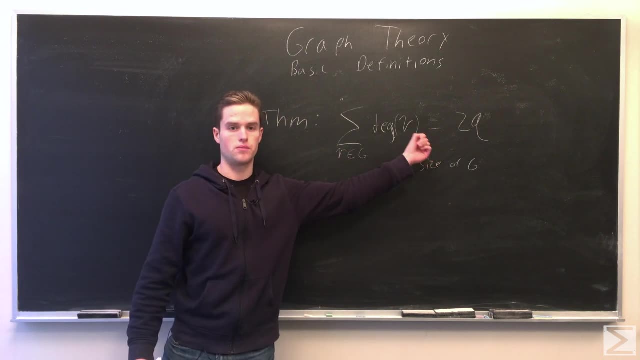 it has this edge relation to. We can prove: if we take the sum of our all V in some graph G, take the sum of all the degrees of V, this will equal two times the size of G, the number of edges in G. 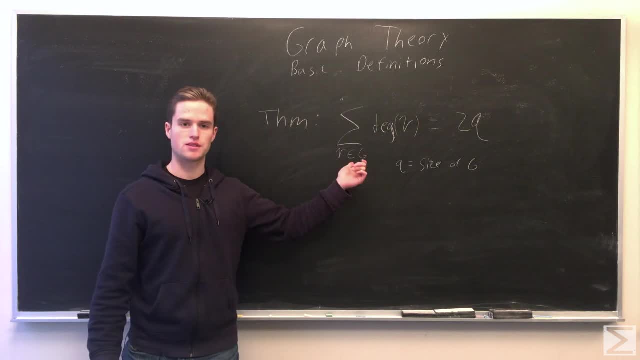 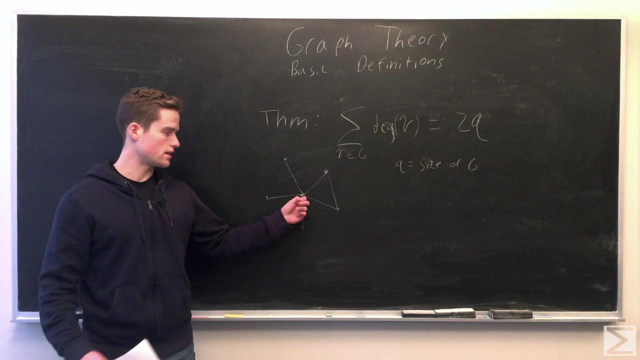 And so this is a fairly simple theorem it comes from. if we add up all the degrees, we're just counting each edge twice. So, like here, the degree of the center vertex is five, the degree of this one, two. As we go through this, take this edge.